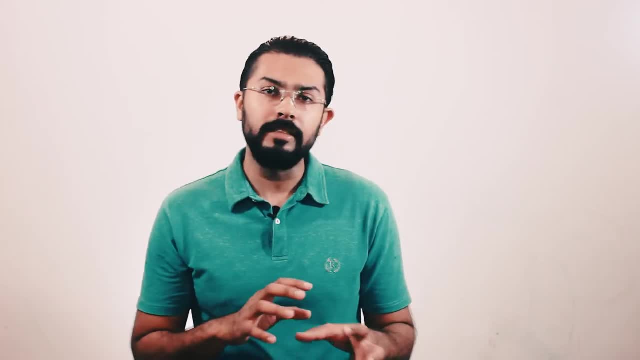 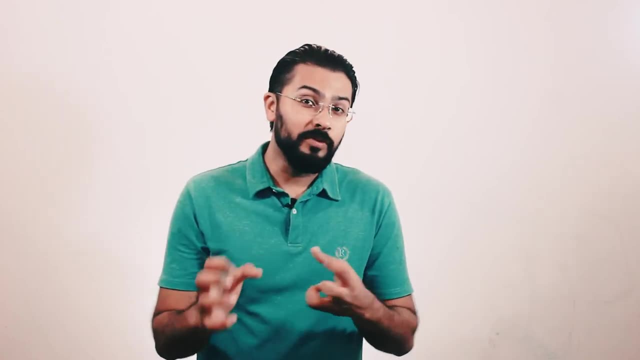 Now the concept of fracture toughness is kind of related to the brittleness of a material. When a material is strong enough to break or break hard, it can give support. That is what we call fracture toughness And impact strength. material is brittle, it fractures sooner, which means it doesn't have the strength. 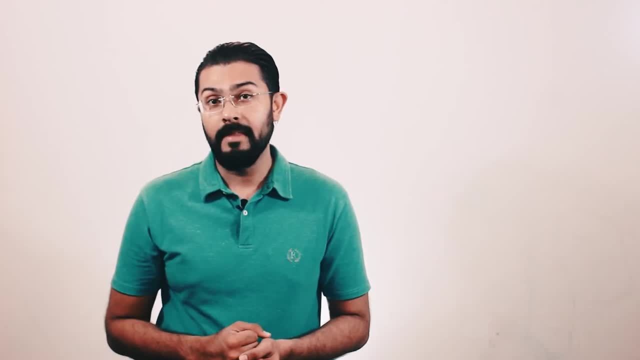 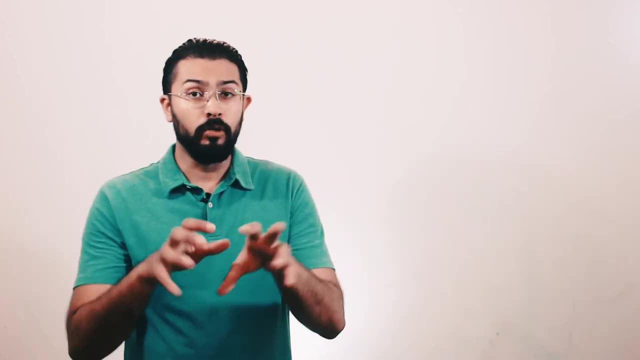 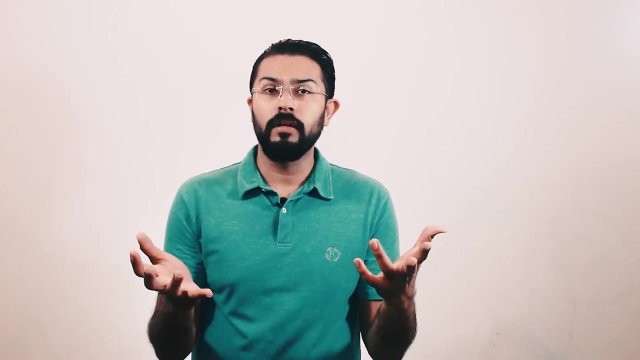 to bear the stress being put on the body. A factor that could make a material weaker is crack propagation at the end of the material when the load is applied. If a material is put under load and cracks are generated, it would fracture very soon, and if we compare it with a material that can resist crack, 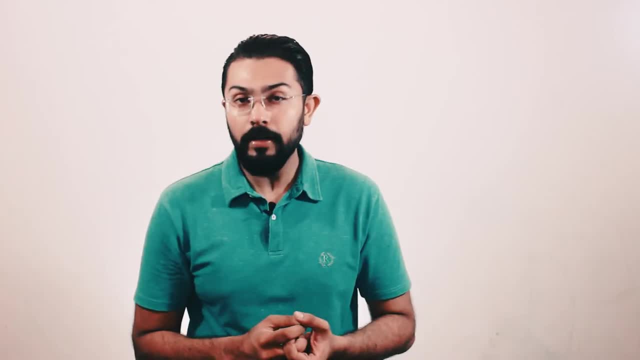 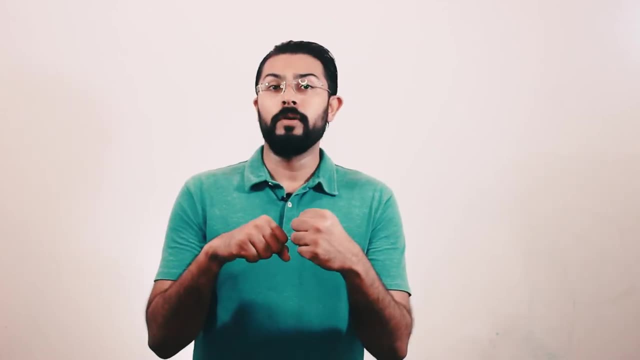 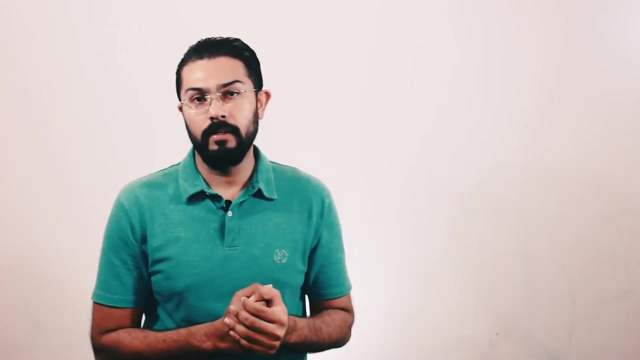 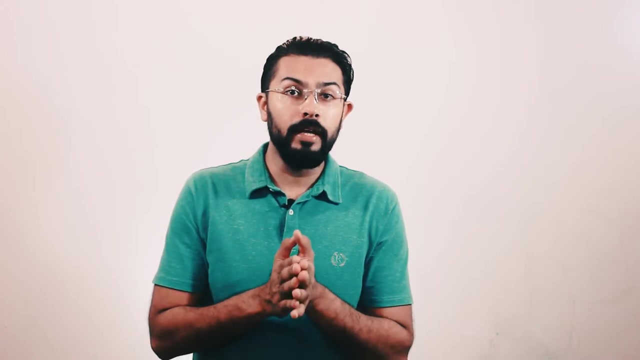 formation under load. that would make a tough material. I hope that's clear now. So basically, fracture toughness is the resistance of a material to fight back the propagation of cracks or to resist the propagation of cracks. If a material has higher fracture toughness value, this means it has the capability of avoiding 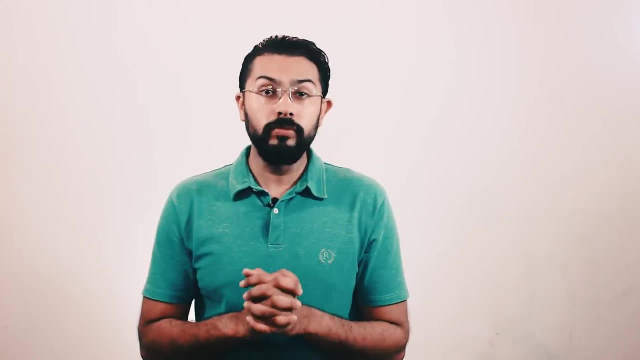 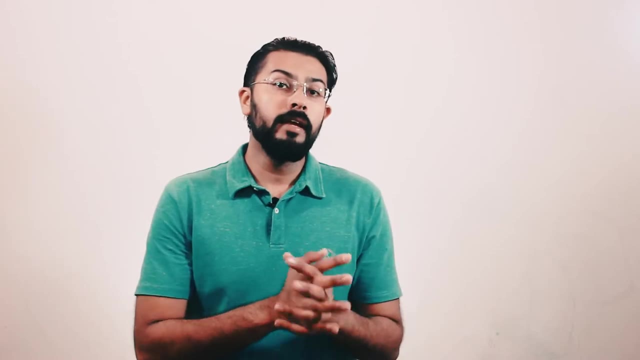 crack propagation and eventually will have more resistance to fracture and eventually will have more resistance to fracture and eventually will have more resistance to fracture. thus it would be called as a tough material. On the other hand, if a material put under load starts generating cracks, would lose its strength too soon and 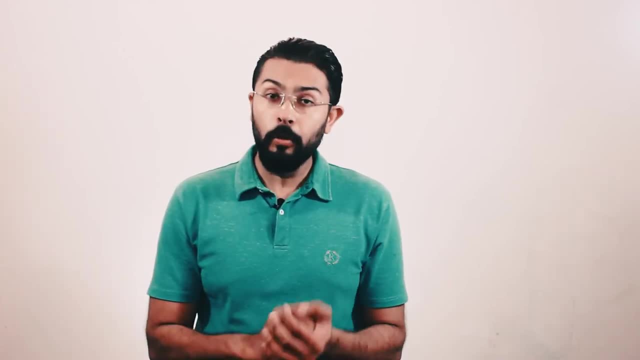 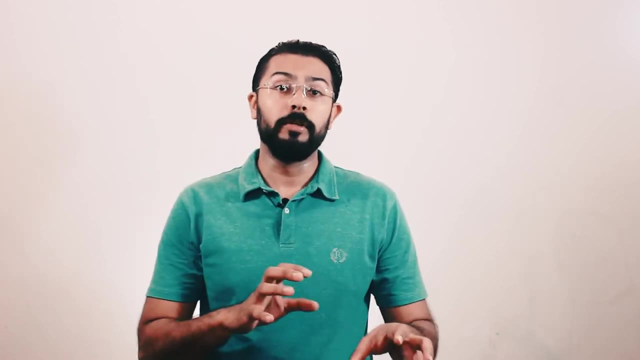 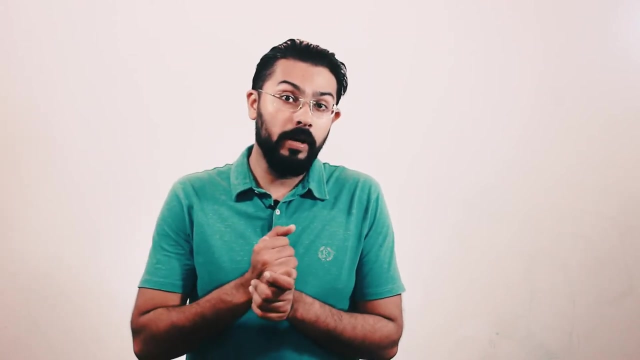 will fracture pretty easily. Now mostly brittle materials are checked for their fracture toughness so they can be handled accordingly. Toughness of a material and crack propagation also have some clinical implications. At a clinic, material could have crack propagation and lose its toughness value due to 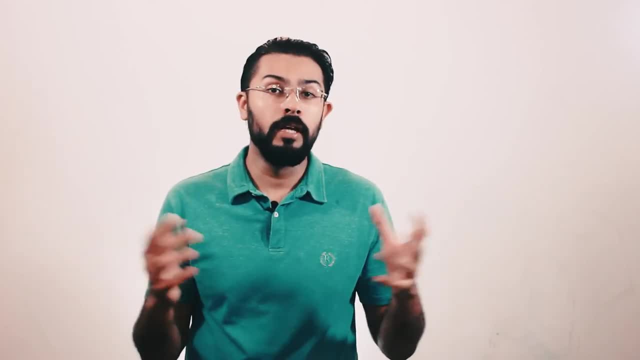 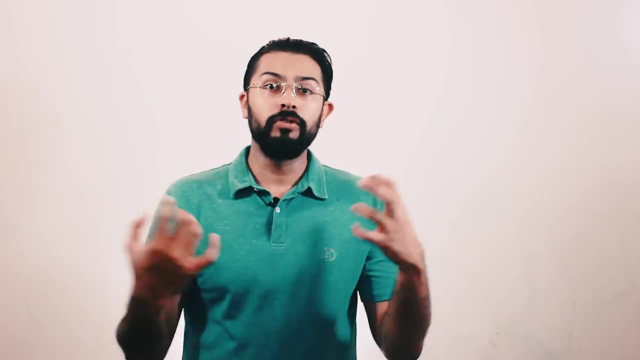 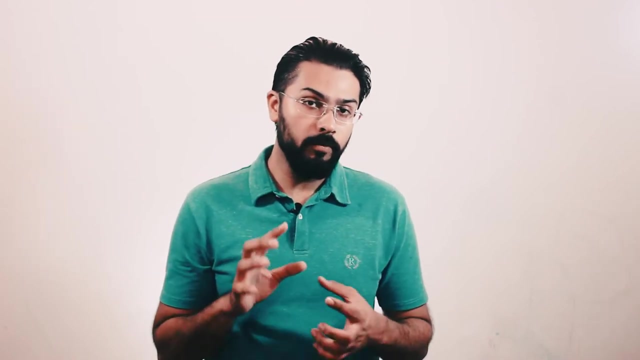 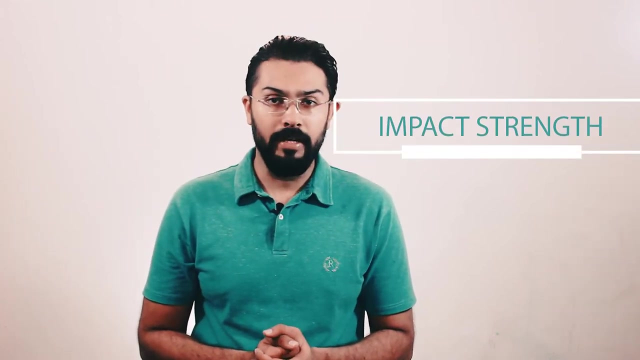 impurities or unwanted temperature and sunlight exposures, or even improper manipulation while mixing, or also due to materials standard physical properties. Now let's talk about impact strength. I hope fracture toughness is clear to you now and you would like to move on further. Let's talk about impact strength. 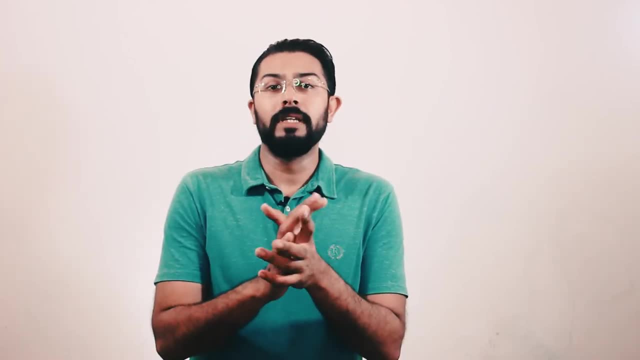 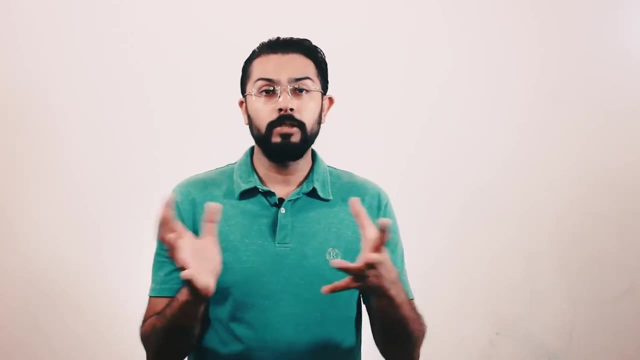 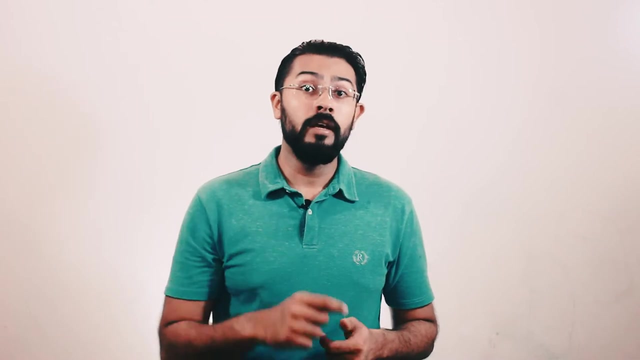 now It is a property which is related to the speed of stress applied. So if a stress on a body is applied slowly, then plastic deformation may occur first, before it reaches to the fracture point. But on the other hand, if stress on the same body is applied rapidly, it might not undergo plastic deformation and 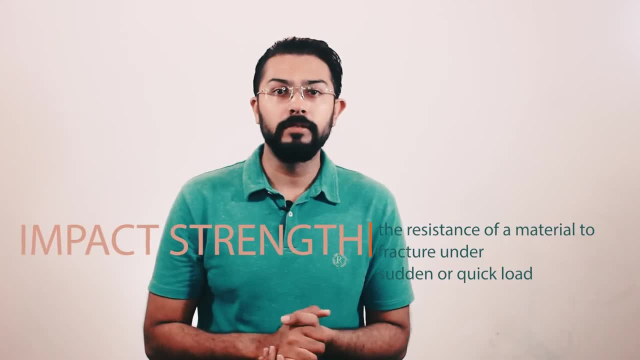 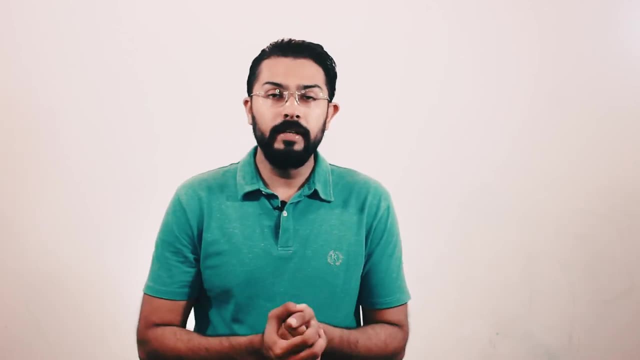 could fracture right away. So the resistance of a material to fracture under sudden or quick load might not be the same as the pressure applied to the same body. So the resistance of a material to fracture under sudden or quickly load is a measure of impact strength. For example, a material would be set to have 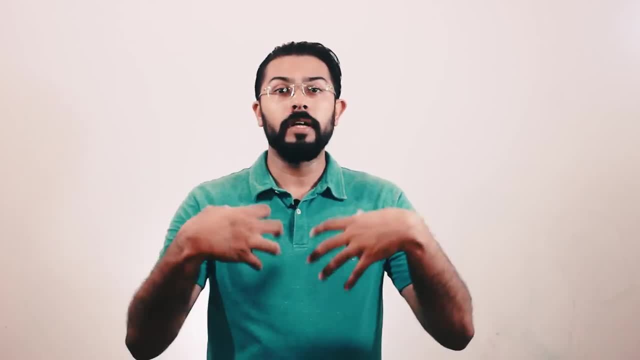 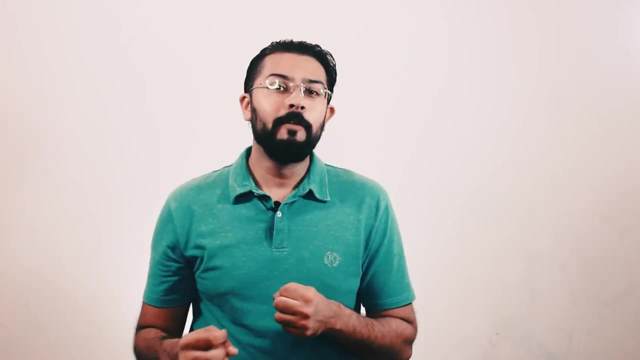 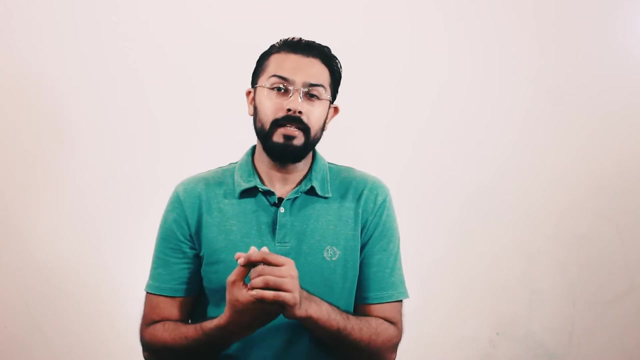 greater impact strength if it can absorb greater energy when undergone sudden blow or rapid load, But a material with lesser impact strength would fracture right after the application of a sudden load. One of the examples of impact strength in a clinical setting is when we talk about the impact strength and 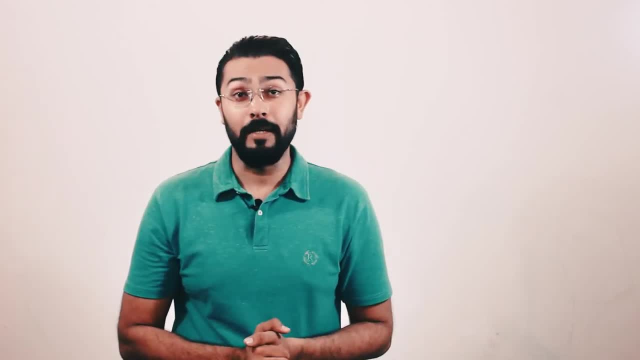 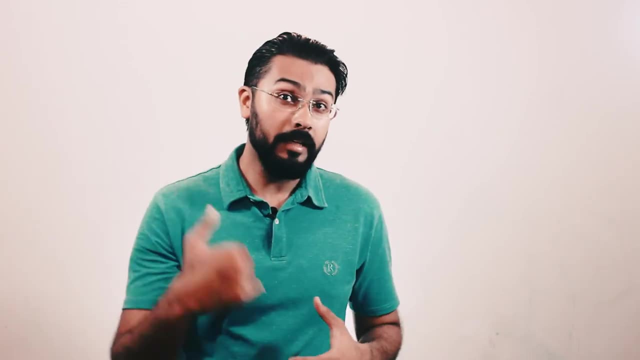 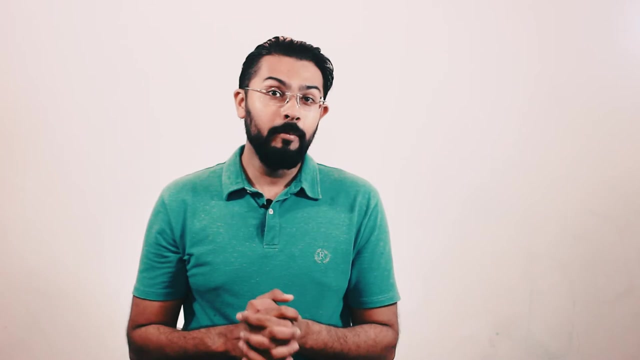 quality of tension, dentures or crowns, For example. if a denture suddenly falls on the floor and breaks, it would have what A higher impact strength or lesser impact strength? It would definitely have a lesser impact strength, right? Because it couldn't. 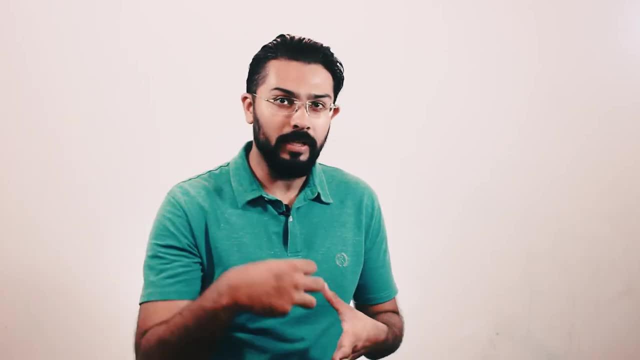 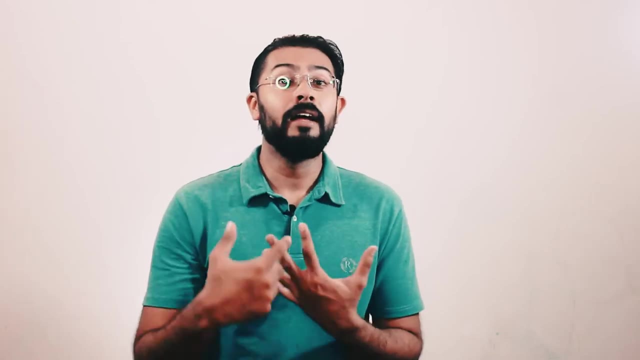 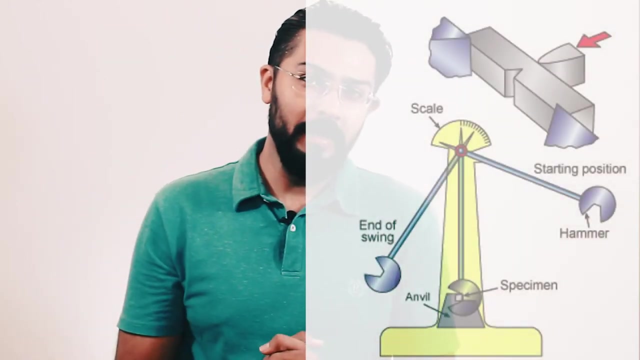 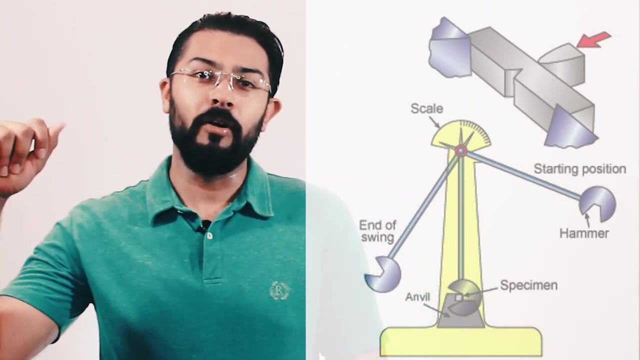 resist the sudden blow or sudden stress that was put on the body. So if a denture is of good quality it should have a higher number of impact strength. Impact strength is tested by a device called Sharpie impact tester, which has a swinging pendulum as an impact tester. So the position reached by the pendulum on 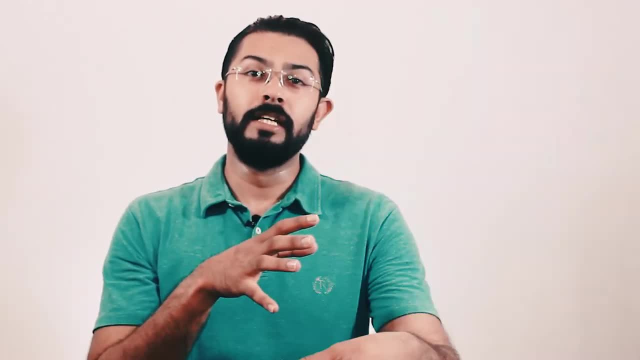 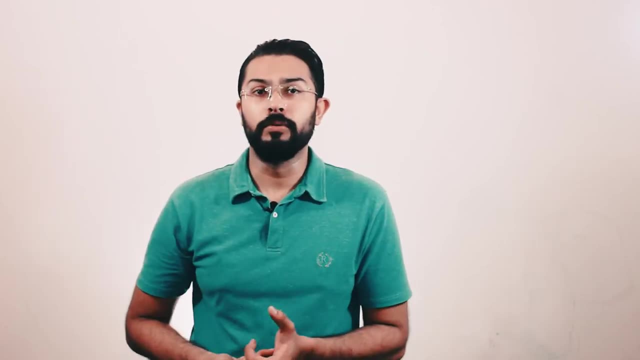 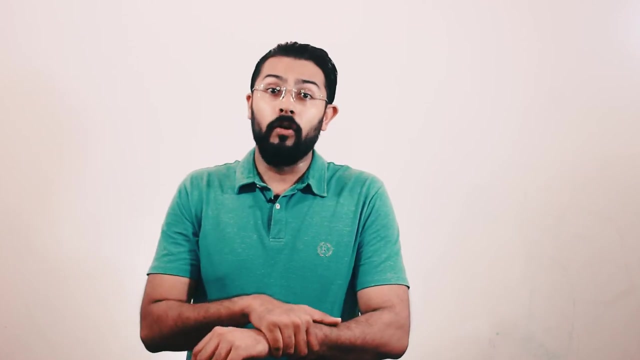 fracturing the specimen gives a measure of the energy absorbed during fracture. Now the measurement that we get from the impact tester also contains the influence of certain factors like air resistance, since the pendulum is swinging in the air, and also friction. So therefore, a dummy run of this device is first done before putting a. 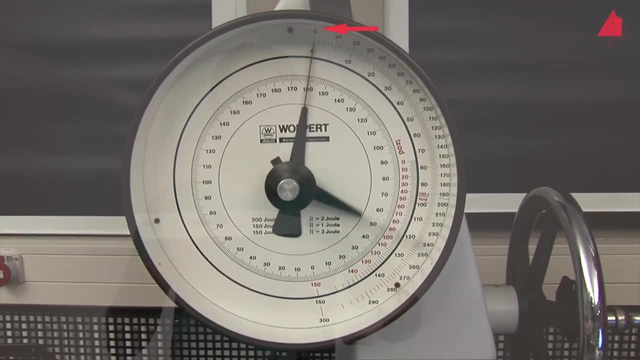 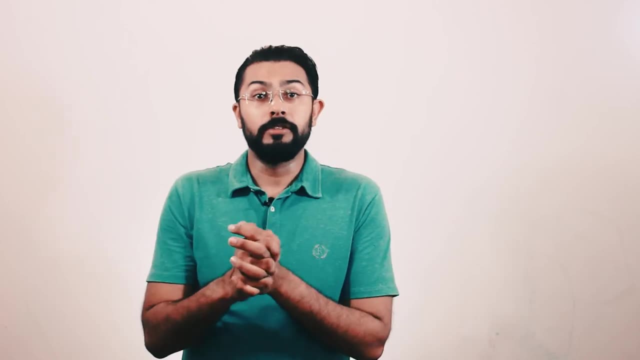 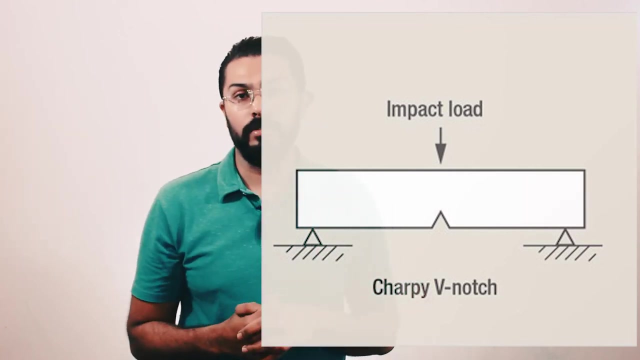 specimen for testing so that accurate readings can be obtained through the test. Okay, and then the specimen is tested in two ways: First, without any cracks or notches, and secondly, by intentionally introducing cracks or notches If the material fractures quickly after introducing notches or 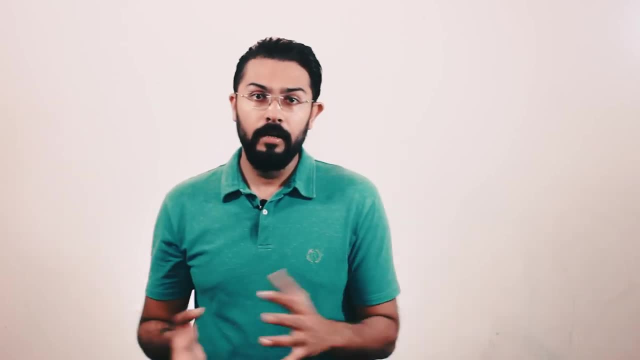 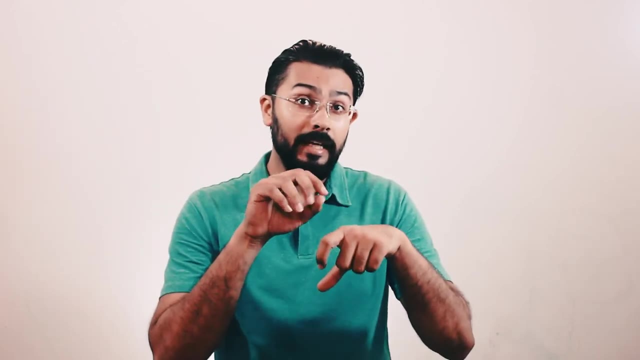 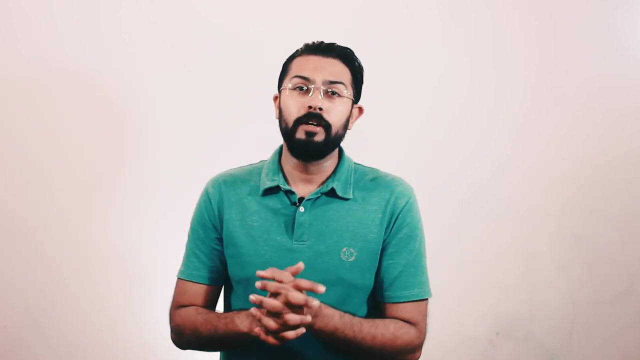 cracks. it is termed as a notch, Notch sensitive material, So notch sensitive material would be a material which fractures too soon after intentionally creating notches or cracks during a during a test. Okay, I think we should end this video here and if you want to go back and revise what we learned,